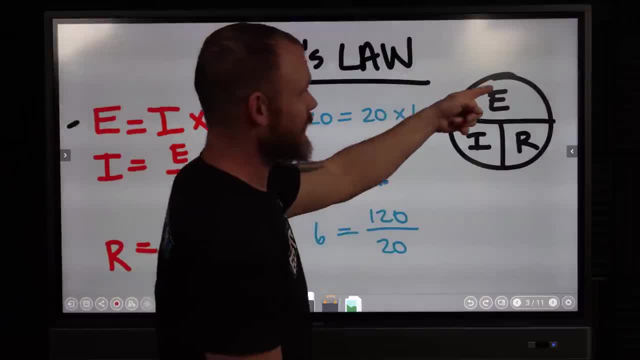 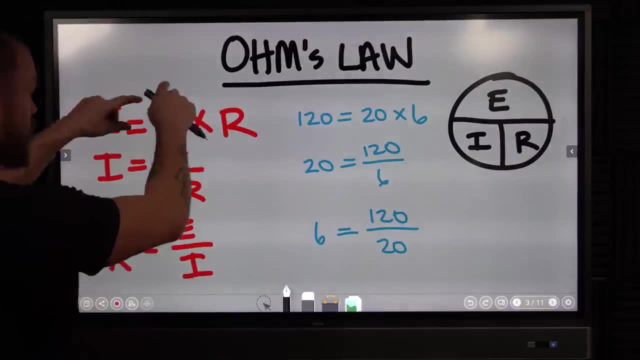 the first one: E equals I times R. If you're trying to solve for voltage, E equals I times R. Just remember they're right next to each other. I times R. If you wanted to solve for amperage, you could sit and try to like divide out the R and move everything over, or you just look at this and be 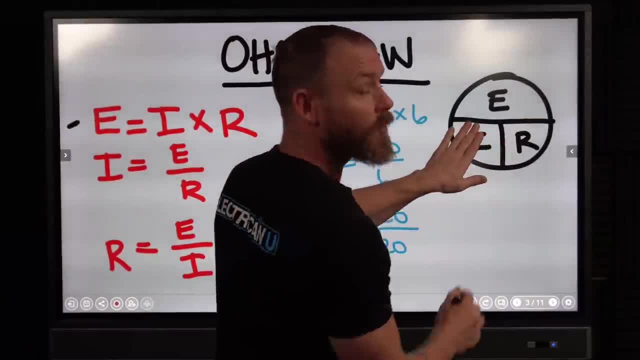 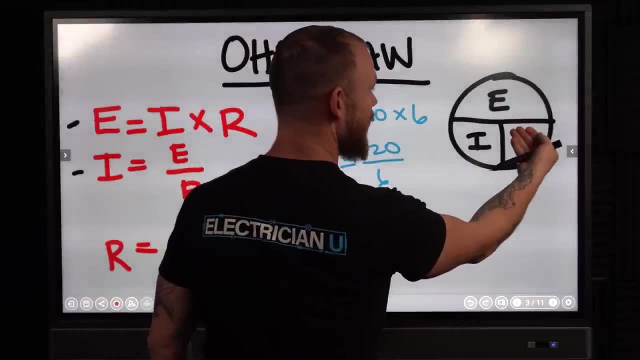 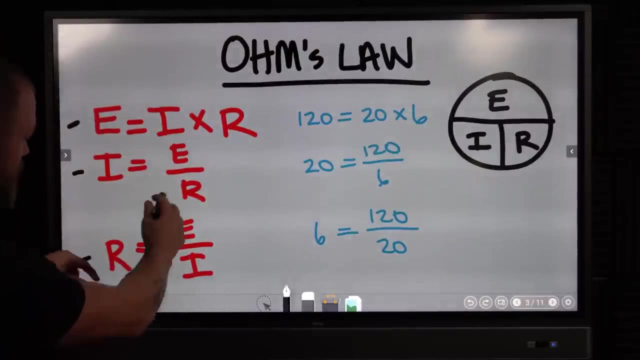 like I'm trying to solve for I, so cover I: it's E over R, So super simple. And lastly, as you would expect, R equals E over I. So that tool, that little chart, is really good, because then otherwise you'd have to like do all of this math and try to multiply by things and like move things around. But if we 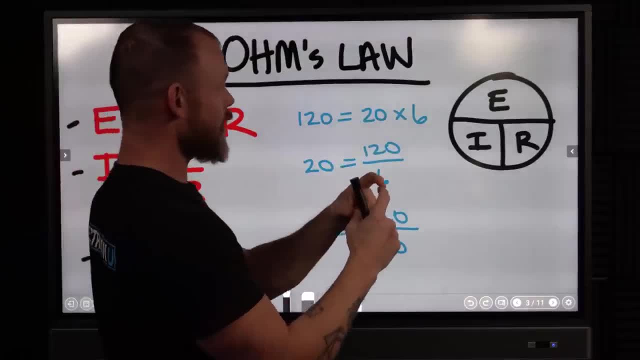 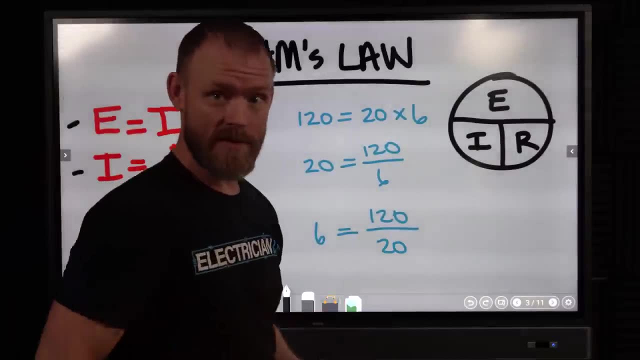 have an amperage that's 20 amps times a 6 Ohm resistor, it's going to be 120 volts. If you're trying to figure out how many amps is it, I got 120 volt circuit and I know this resistor is 6. 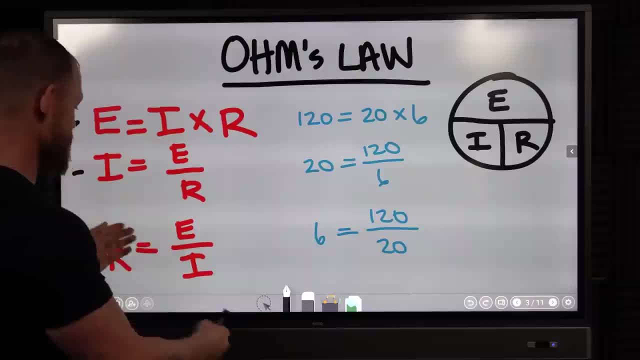 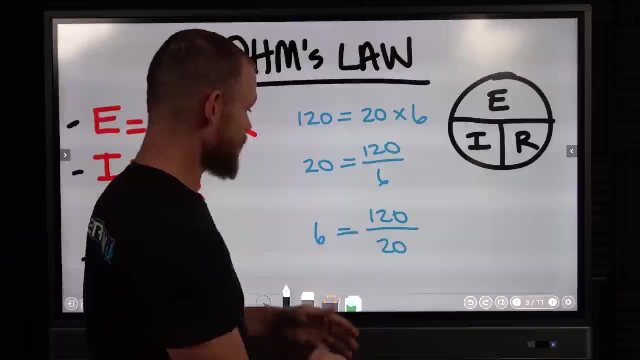 Ohms, You just divide and you get 20 amps. But if you don't know what the resistance is of a resistor, But you know that this thing is drawing 20 amps and it's 120 volt circuit, You can just divide that and figure out 6 Ohms. So this is a really really helpful thing to use. Next is going. 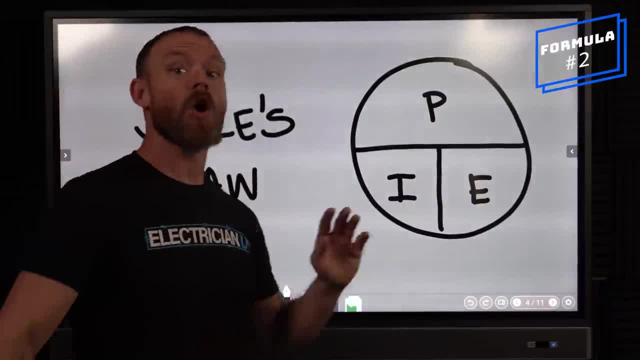 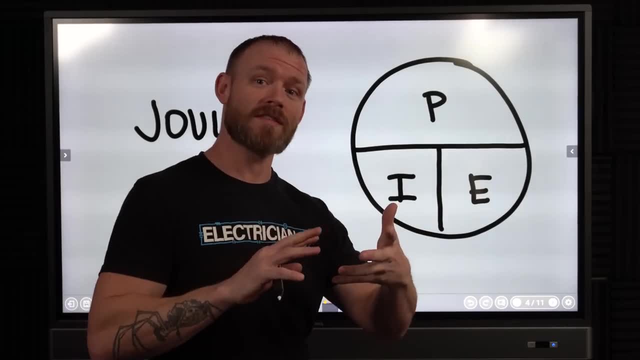 to be Joule's law, So a lot of people don't call this Joule's law, but that's what it is. Joule's is the amount of energy that's produced by something or that's transferred from one system to another system. So when we're talking about electrical energy going through a light bulb, we're talking. 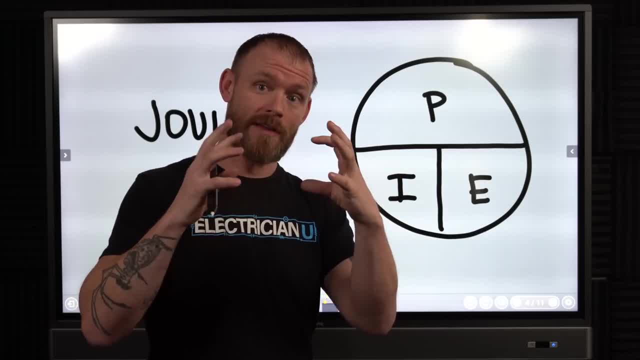 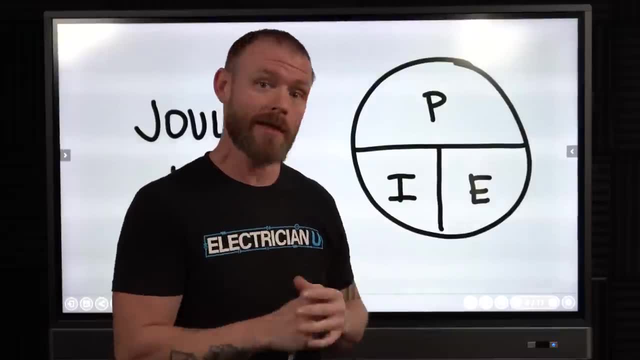 about the amount of energy that is coming from the electrical system. So when we're talking about electrical energy in the electrical circuit and that is being produced or transferred into another kind of energy, like light and heat in the case of like an incandescent bulb, So Joule's law, 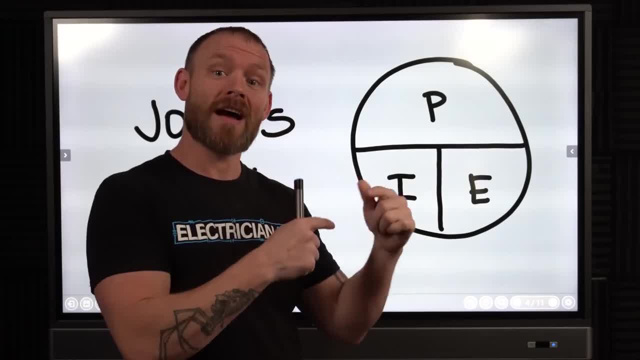 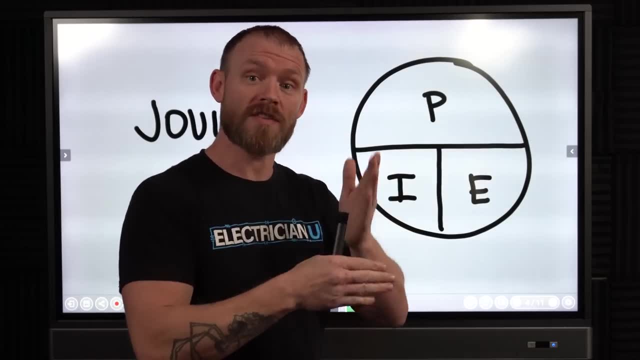 is usually a function of time, So usually in a formula they're going to have time as a function. but amperage includes time, So amperage is a rate, So it's current, that's flowing per second, So it already factors that in, So we can call this Joule's law and use it as such. So very similar. 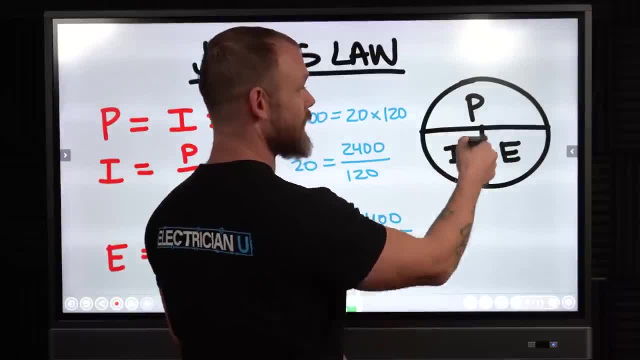 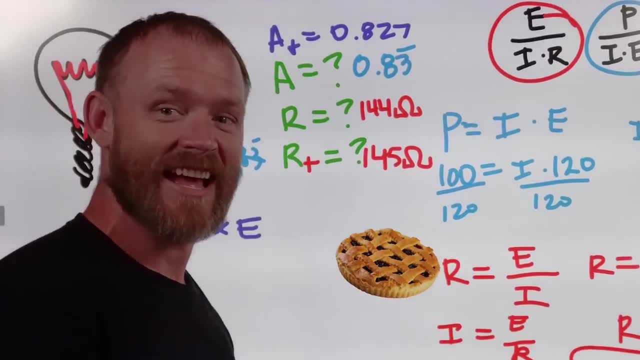 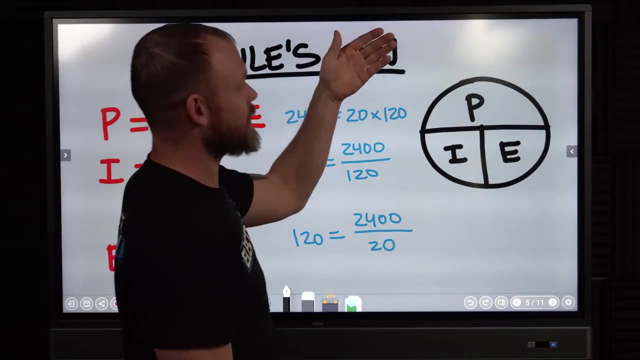 kind of thing. instead of E equals I times R, Now we have P equals I times E. I just think of pi, Yummy pi, P-I-E Pi. That's how I think of it. So the one thing if we're trying to solve for how many, 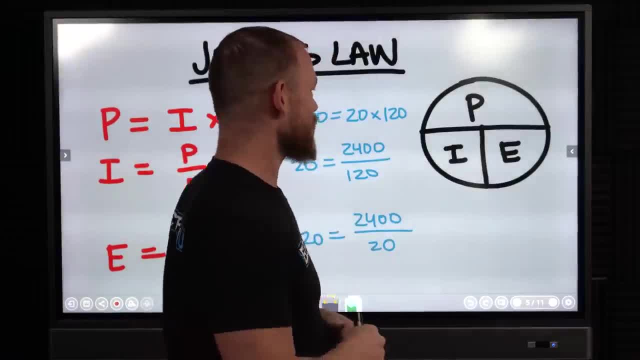 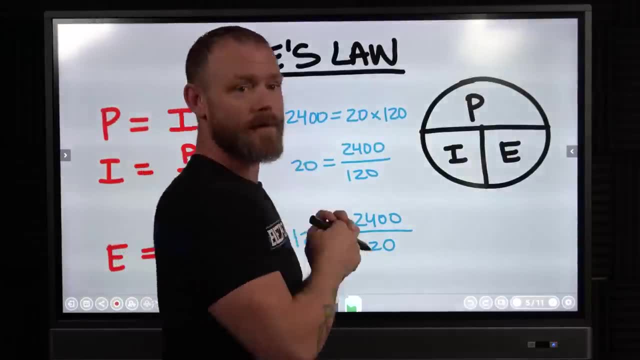 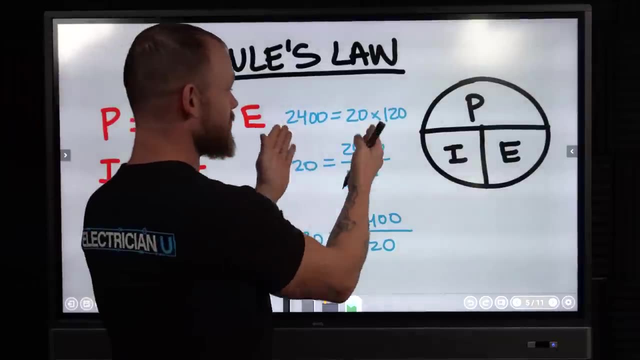 watts of like light bulbs that we have. What's the total wattage of a circuit once we turn all these bulbs on? Well, we know it's a 120 volt circuit and we know that it's drawing 20 amps. So how much total power is that? It's going to be 2400.. So we could take all of these values and 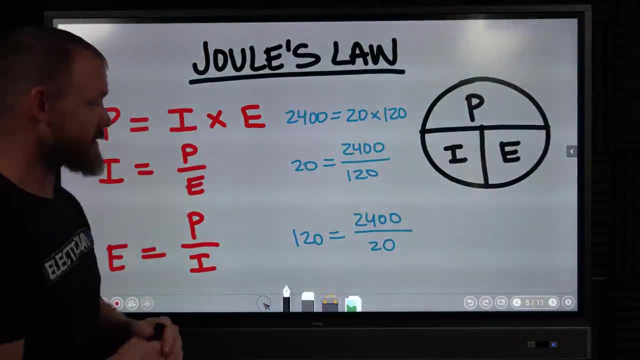 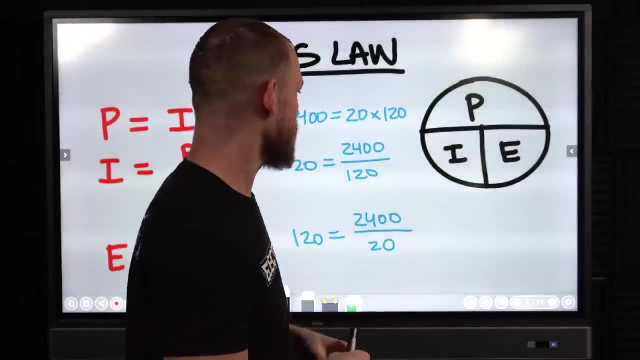 the same thing. All of them are true. If we're trying to figure out how much current draws in a circuit, well, we know we have 2400 watts in a circuit and say we're trying to figure out like a 20 amp breaker, You know 20 amp circuit. Well, if it's 2400 watts that we have to deal with, 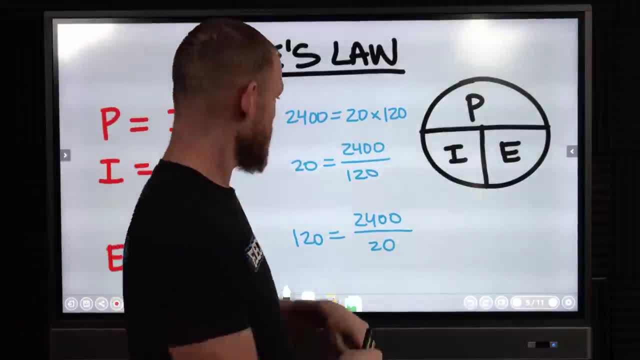 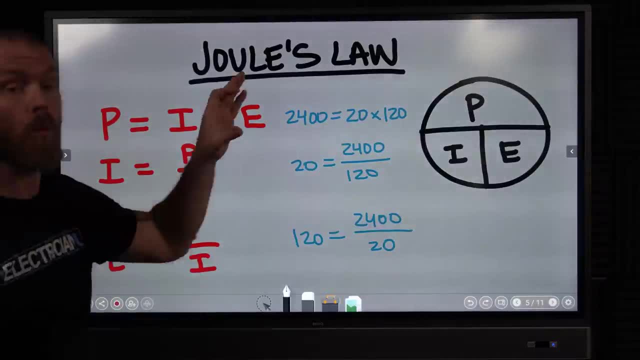 divided by 120, then that's going to be 20 total amps for that circuit. You could also do the inverse, So say that we're trying to figure out for what the total wattage of a circuit is. if we have a 20 amp breaker, 120 amps, then we have 2400. 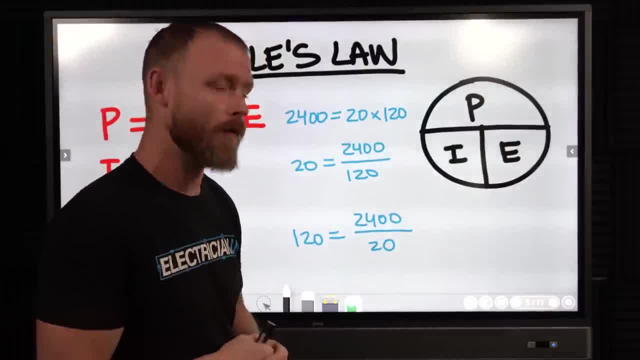 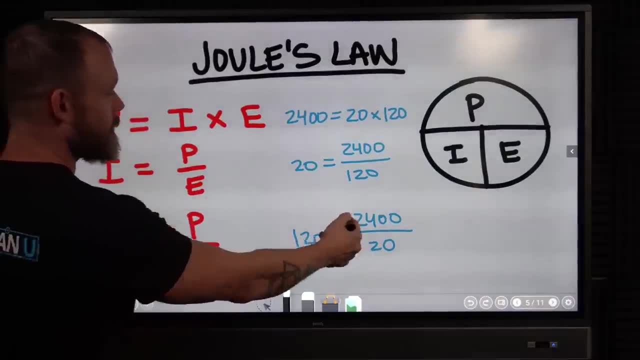 watts to play with in a 20 amp circuit. That's another like helpful thing out in the field. So anyways, lastly, if we're trying to solve for voltage- which you're never going to do- you're going to take the power, whatever the the wattage is. divide that by 20 amps if you're. 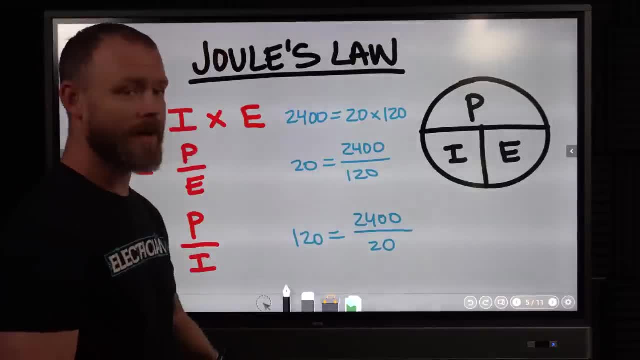 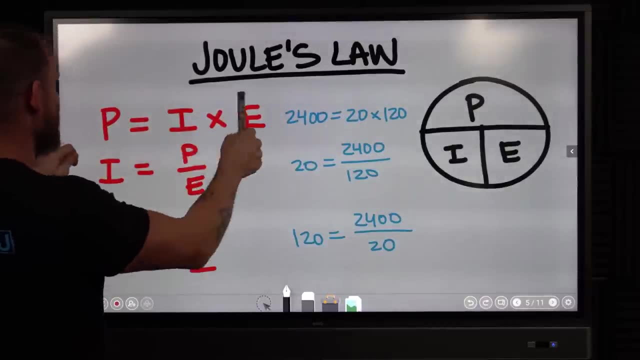 testing 20 amps and it should be 120 volts. So they all organize nice and neatly. Again, rather than doing the math to try to figure out what the total wattage of a circuit is, You're going to have to figure it out and like divide by e to isolate i and move e over. here You'll have to. 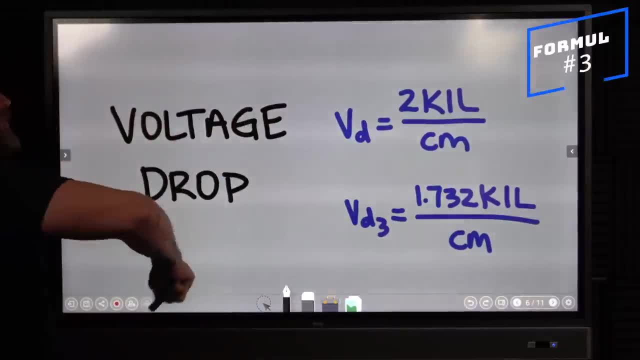 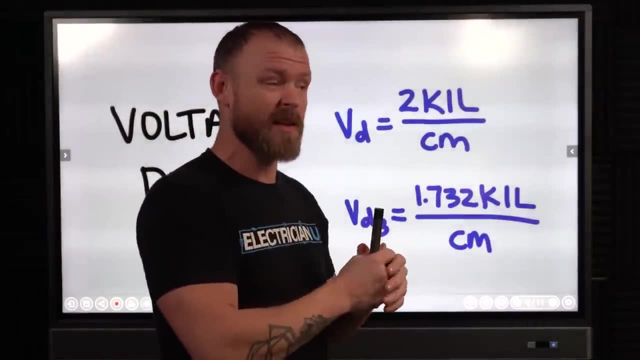 remember all that. Just remember the pie chart. Next up is voltage drop. So voltage drop is something we're very frequently going to come across in the field. You can actually use Ohm's law to do a voltage drop calculation without all the extra variables. It's just slightly off, It's. 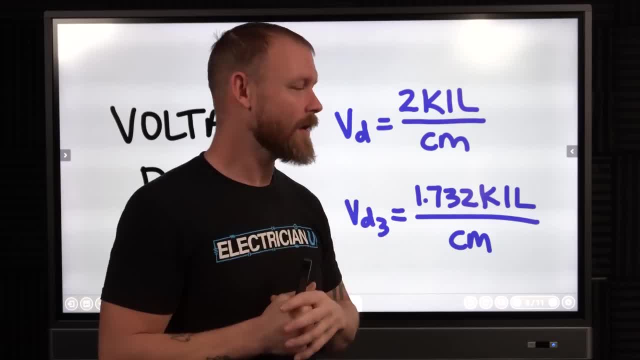 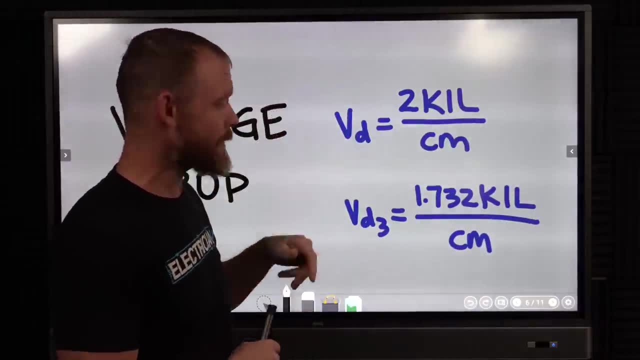 not going to be as accurate but kind of like, gets you relatively close. But a better way to do voltage drop is to actually use voltage drop formulas. You know I have two here. One of them is this one called VV3 and it's a VD3 formula. VV3 is voltage drop, The other one is VV3.. 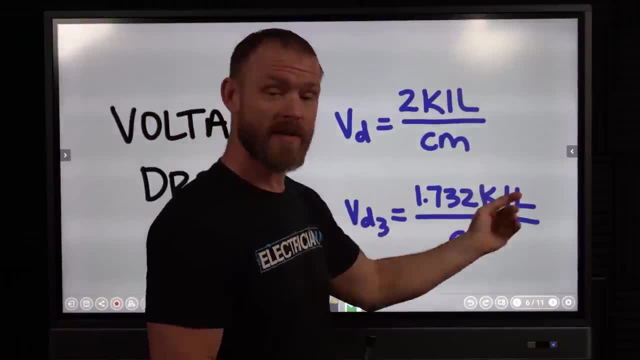 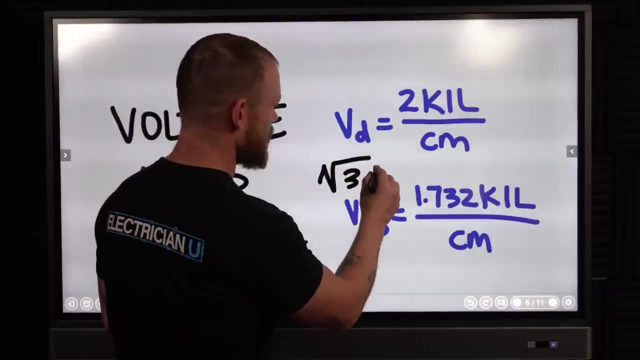 For three phase. So anytime you do three phase, you have to introduce 1.732 into the formula. It's also the square root of 3.. So the square root of 3 equals 1.732.. So you're going to notice. the formulas then are very similar. One of them is: 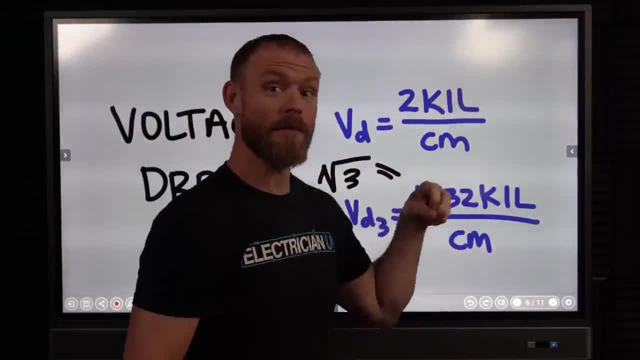 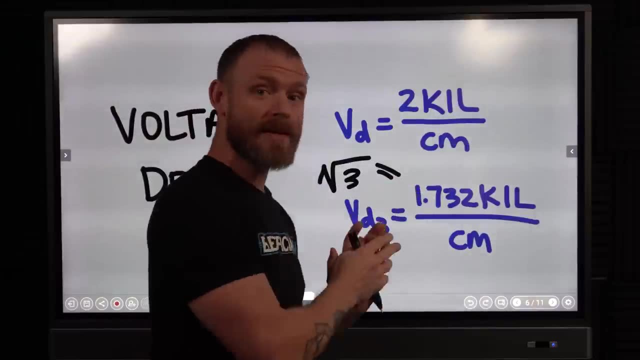 two times a bunch of craziness. The other one's 1.732 times a bunch of craziness, which that means this is a smaller number. you're multiplying by So that typically in a three circuit there's going to be slightly less voltage drop. Voltage drop is more expressed in a single. 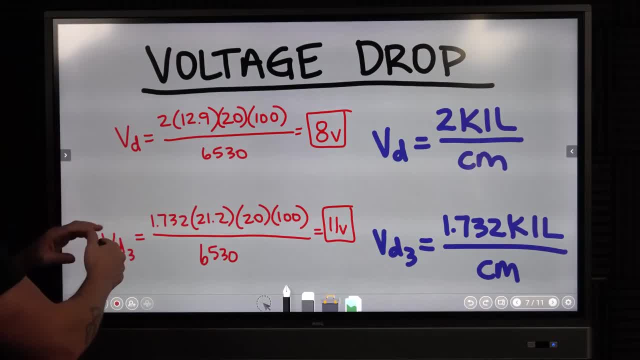 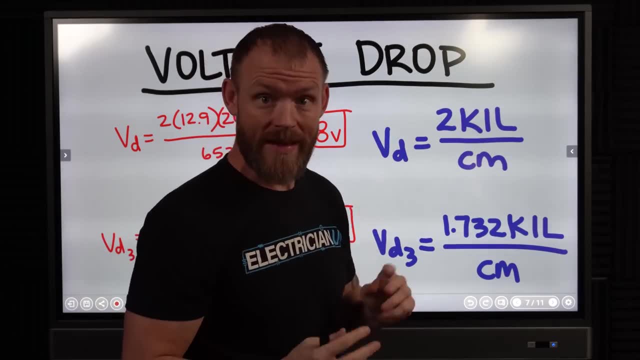 phase circuit. All right, So voltage drop. let's do an example. So the two, I think of it. there's two conductors, right, You have there, and back We have length which is L, So if you have a hundred, 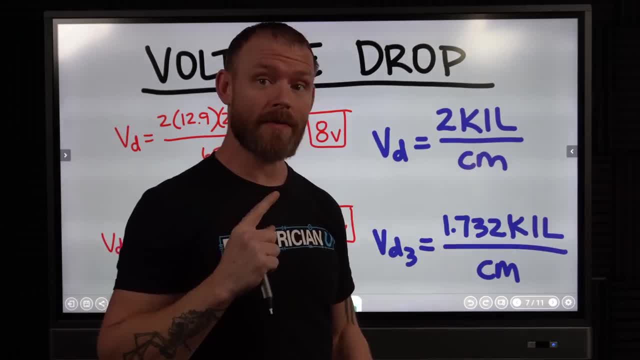 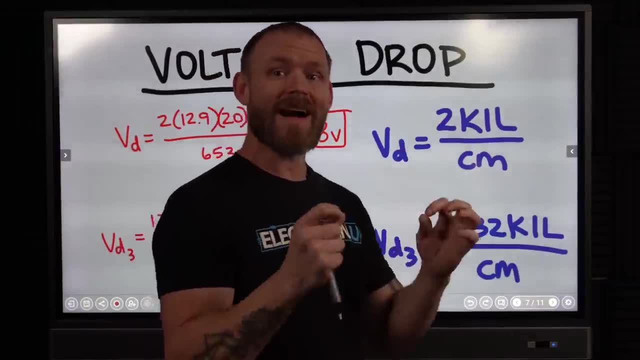 feet. you're not going to measure a hundred feet one way and a hundred feet back the other way. That's what that two is for. So the two, two conductors at a hundred feet. that's how I remember the two and the L. The K is a constant that we use depending on the type of material. 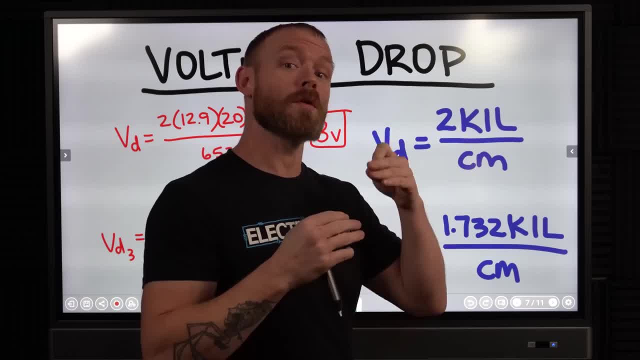 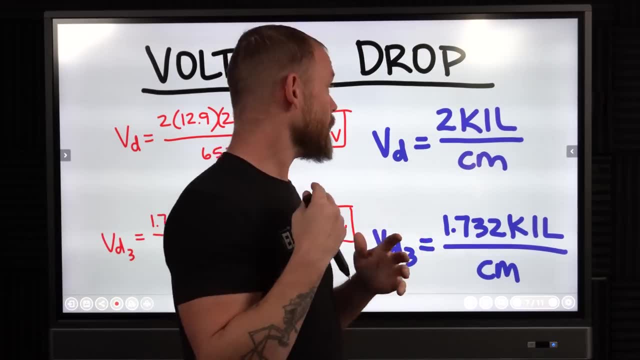 that we're using. So if we're using a copper conductor, the conductivity or resistivity of a certain conductor is going to be different. So aluminum is a little bit less conductive than copper is. So copper you're not going to experience as much of a voltage drop as you are. 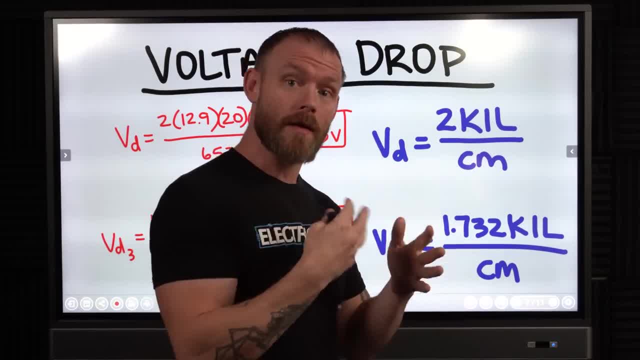 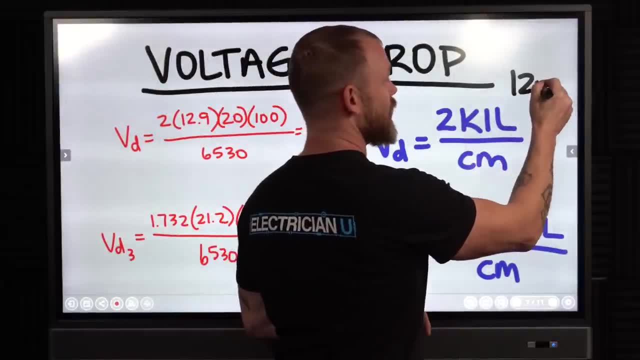 for the same size conductor in aluminum just because they don't conduct as well. There's just more resistance with the material. So K. the coefficient for K for copper is 12.9.. So every single one of these that you ever do, you're going to use 12.9 for copper. 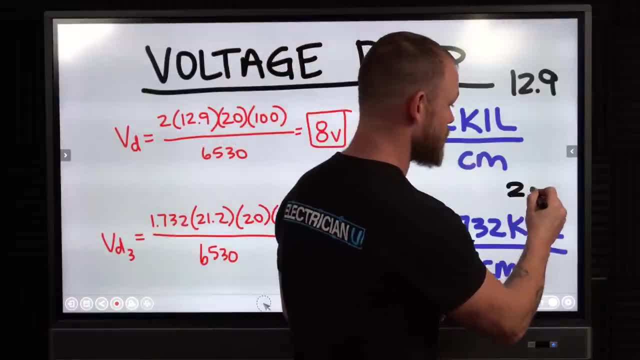 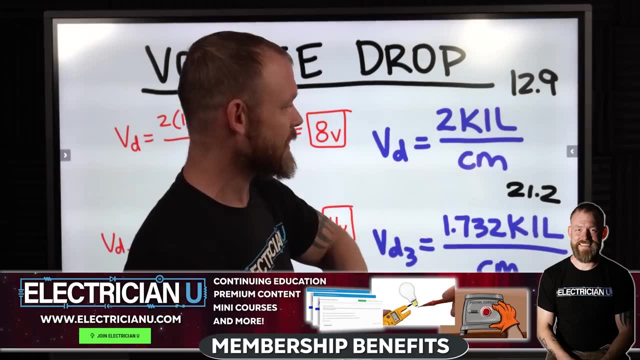 If it's going to be aluminum, K is going to be 21.2.. So just memorize those two numbers and never forget them the rest of your life and you'll be fine. So anytime you're doing aluminum stuff, use that. Anytime you're using copper, use that. So that covers the two. the K I is your amperage. 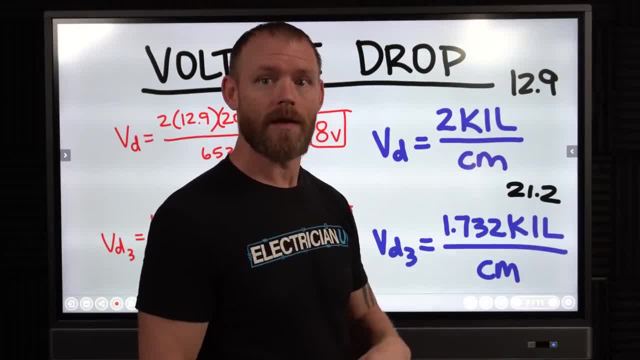 How, like if we had a motor or something that's a 20 amp motor out in the field, you're going to plug in whatever that is going to be. So that takes care of everything that we're doing. So that's the two. the K I is your amperage. 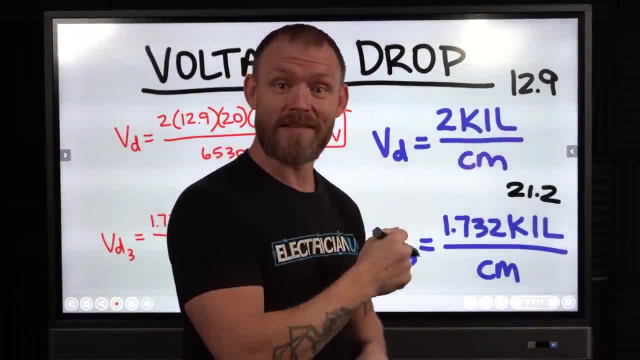 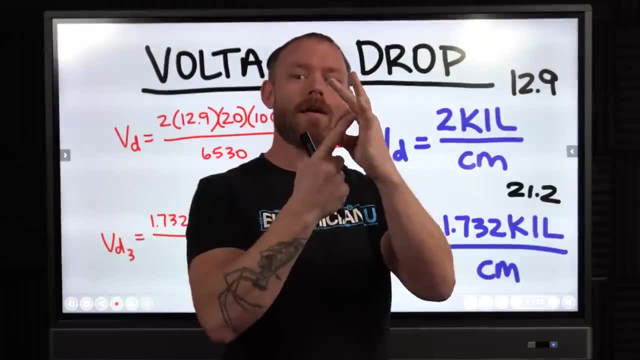 On the top. the bottom is not centimeters, It is circular mils. So every conductor has a certain diameter, which means it also has an area, And the area of that conductor, or the cross-sectional area. if you slice the thing in half, the cross-sectional area of it is measured in. 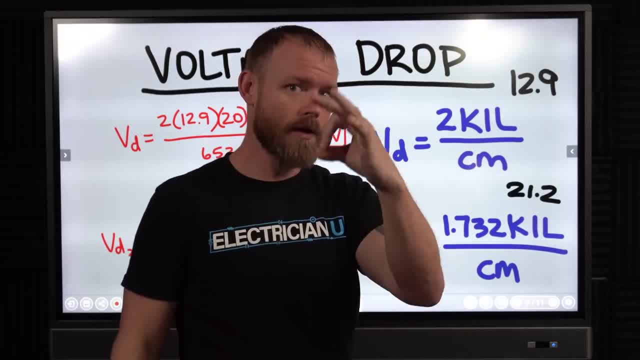 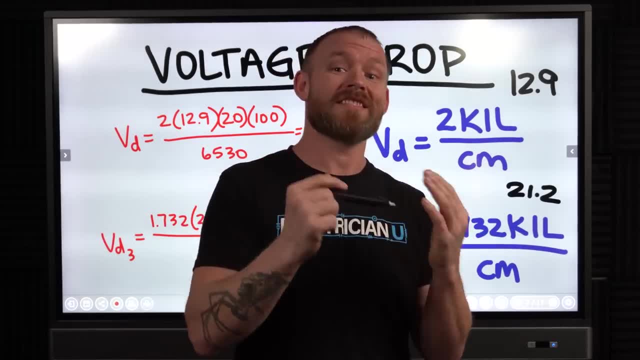 mils or circular mils. So a circular conductor is going to be circular mils, So every conductor has a certain size circular mils. Number 12, I know, for 20 amps, is going to be 6,530.. Just remember that. 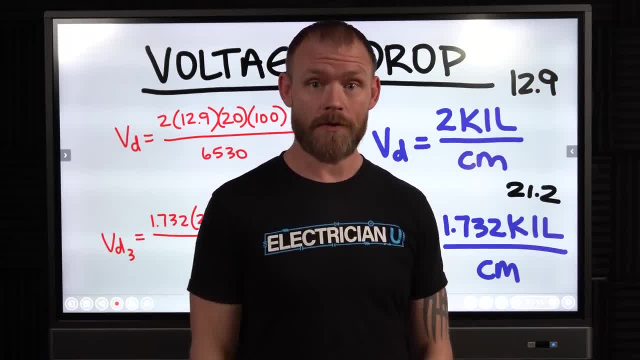 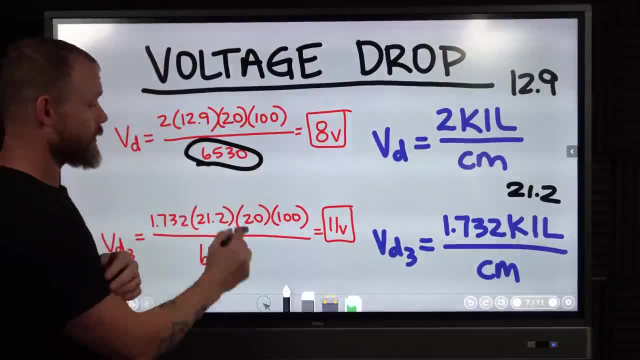 Remember that number because most of the time you're going to be dealing with number 12 conductors and trying to see what the voltage drop is on that sized conductor. So the cross-sectional area of number 12 is going to be 6,530.. Now one thing to keep in mind. 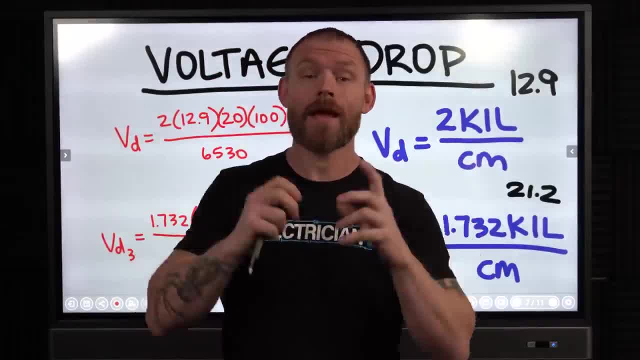 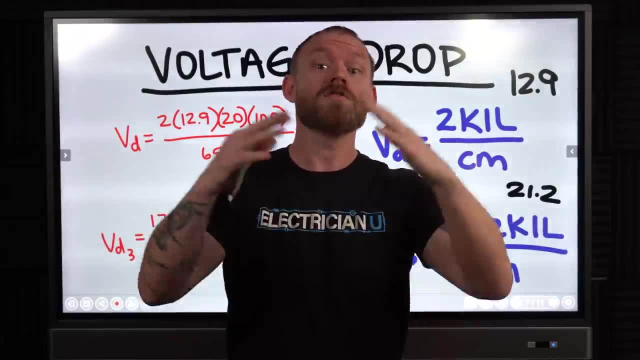 if you're ever dealing with like 250 KC mil or 250 MCM or like 500, 600, you're talking big conductors. the 600 actually means 600,000 circular mils, So those are really easy Once. 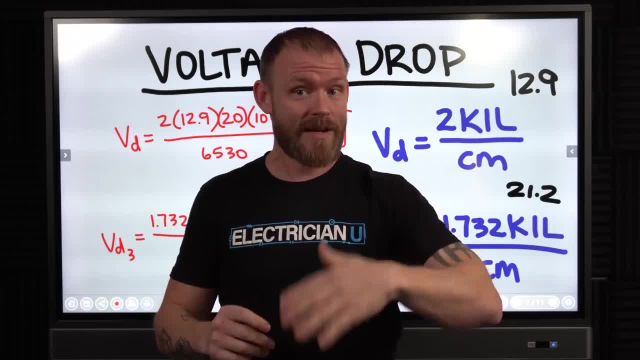 you get past 4i, you start 250,, 300,, 350, all of that. That's actually talking about the circular mils, So that's really easy. Once you get past 4i, you start 250,, 300,, 350, all of that. 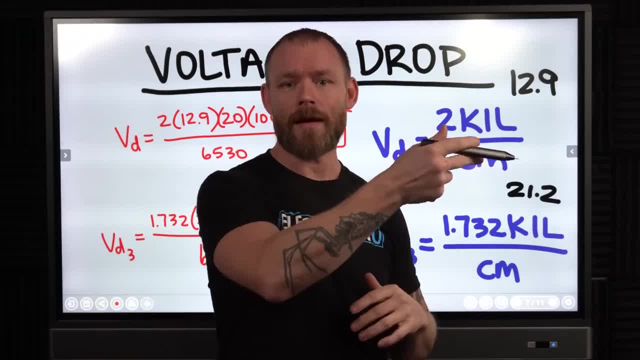 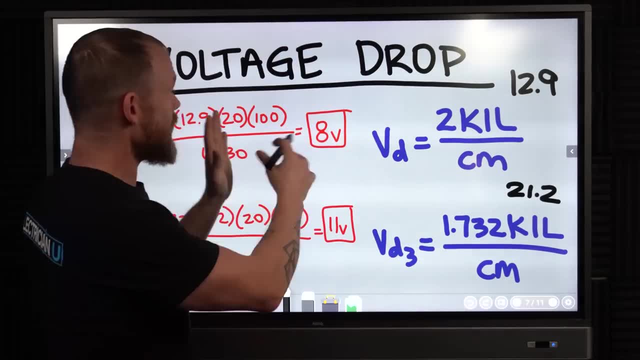 That's actually talking about the circular mils. So otherwise, chapter nine, table eight, NEC, it's going to have all of these values in there for each specific one. So beyond all of that, like that's what we're plugging into the formula. So an example is: say we've got a single phase. 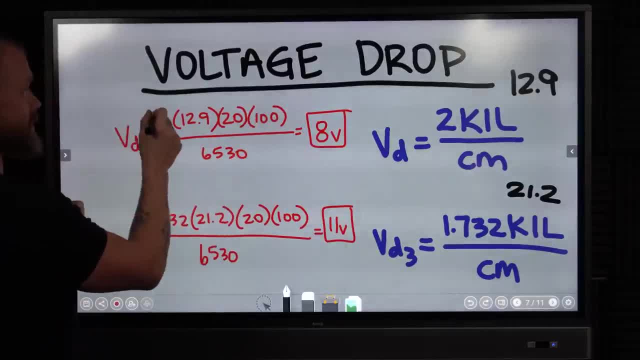 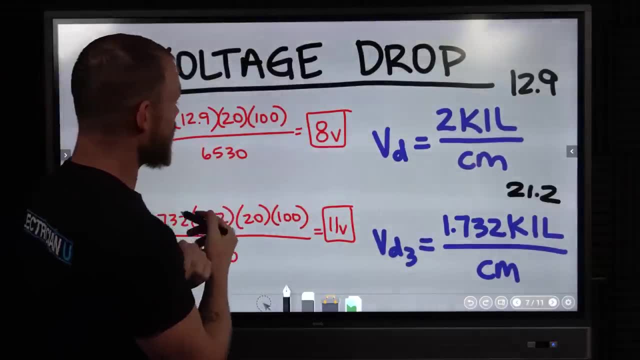 voltage drop that we're trying to calculate. We've got a hundred foot distance. There's two conductors, they're copper, So it's 12.9.. It's a 20 amp load divided by number- 12 conductors, which is 6,530.. We get eight volts. So in this situation, 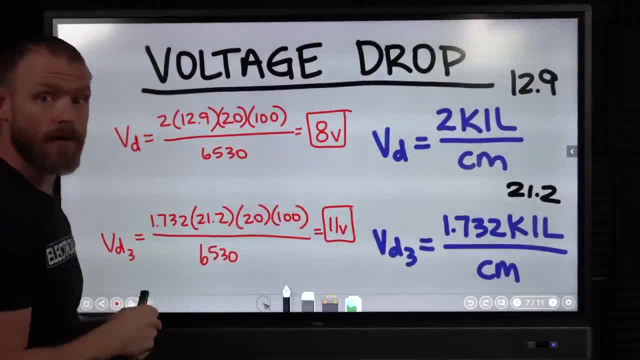 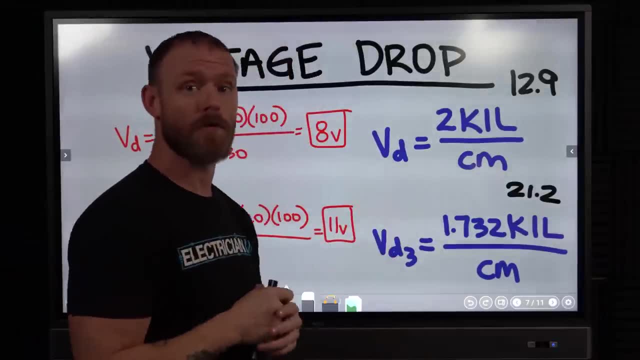 if we have a hundred feet, if we have a 20 amp motor on copper conductors- that's number 12, we're going to experience an eight volt drop. when we hit that thing and actually start it up, it's going to drop the whole voltage of the circuit. Now for three phase again. 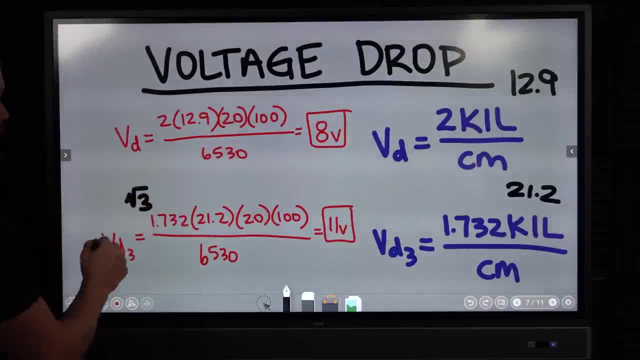 we see this 1.732 thing square root of three, right, Because it's three phase, So everything three phase. we've got to add this 1.732 thing, So we have square root of three times 21.2. this. 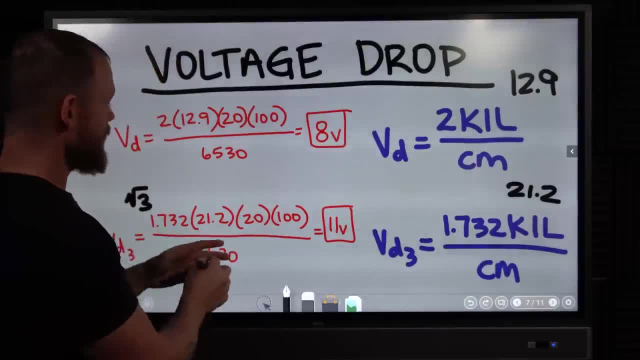 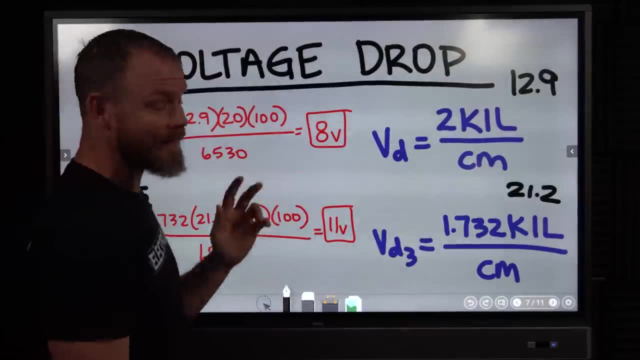 time, instead of copper we're going to say we're using aluminum, just to see what that does. Still, the 20 amp load is still a hundred feet away and we're still using number 12.. It's just number 12, aluminum this time. Do all of the math and we figure it's an 11 volt drop. So other than we? 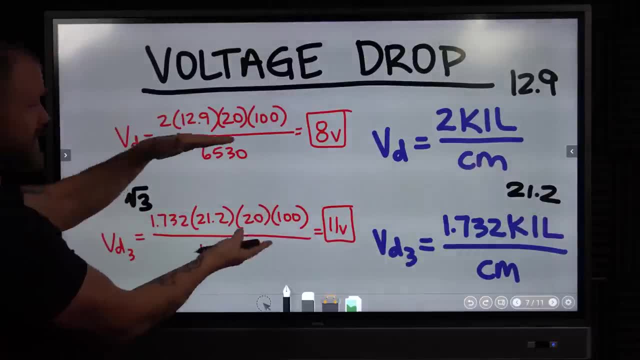 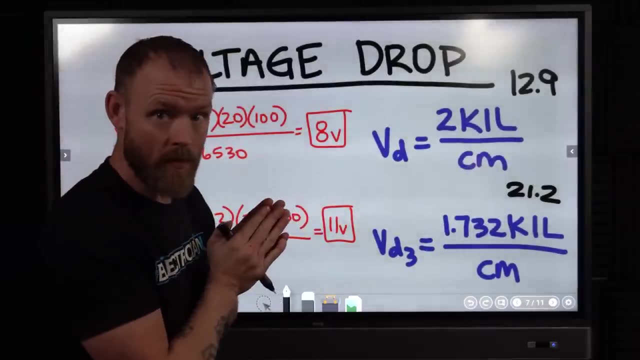 changed and put 1.732 instead of two. this voltage drop if it were both single phase, just changing the aluminum conductors- would have still made this thing drop a lot more volts. It's actually less of a voltage drop because we're in a three phase circuit. So 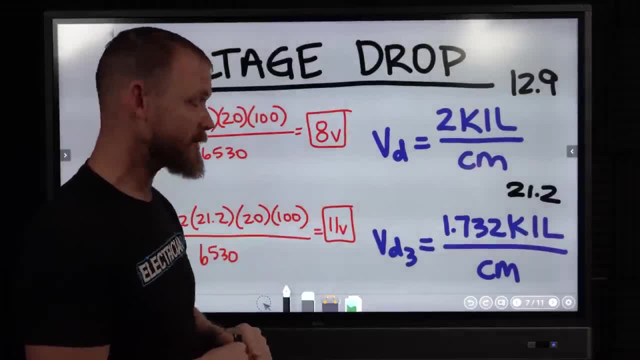 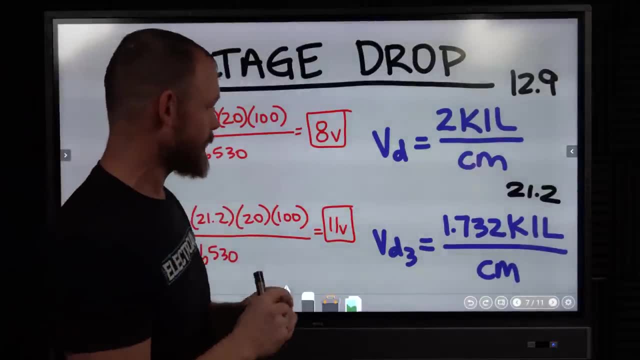 it would probably be higher, maybe 12 volts, if we were just doing single phase. but even when you go up in aluminum for that higher coefficient, you go down because it's three phase, just slightly Next up. you're going to see this on every damn test, you're. 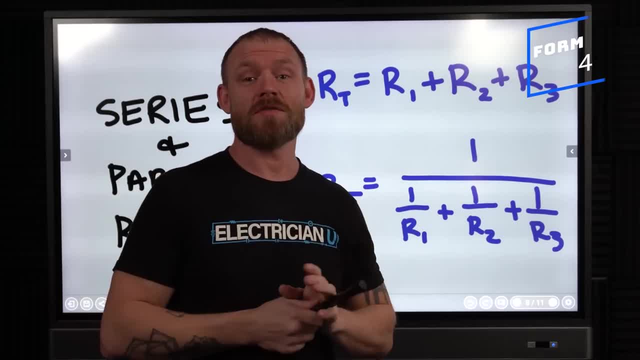 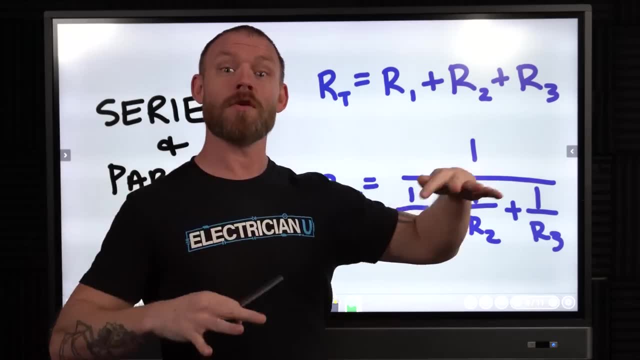 ever going to take electrical theory. This stuff sucks, especially once you start getting into RLC circuits where you've got resistance, inductance and capacitance in series and in parallel And sometimes, when you're doing capacitance, these formulas for capacitance. 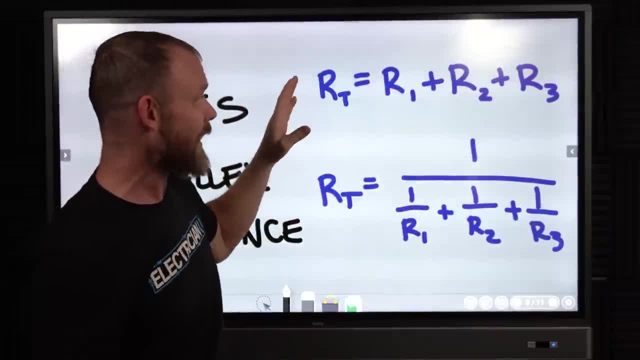 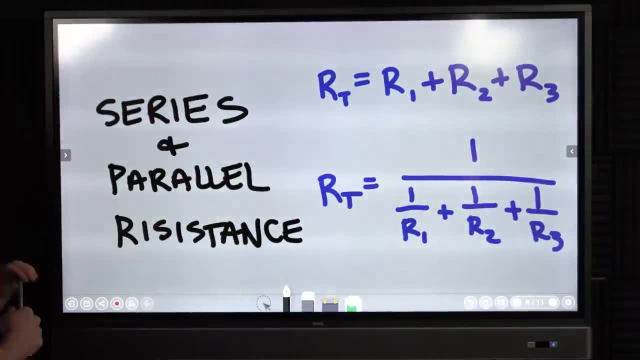 are actually completely inversed. So capacitance in a parallel circuit is going to look like this. capacitance in a series circuit is going to look like this, But not to digress series and parallel resistance. if you're trying to figure out the total resistance of a series circuit, you just add: 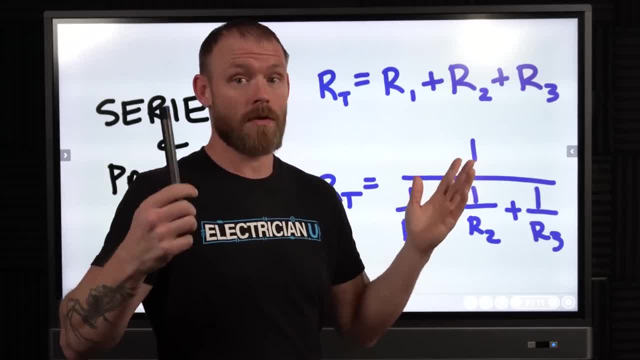 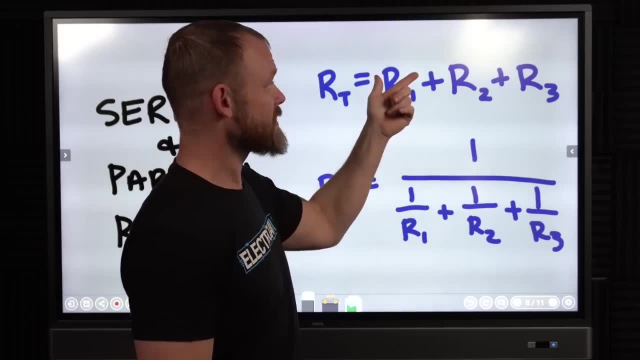 all the resistances together. It's the sum of all of them. It's super easy to do. You're in series, you're just adding one after the other. So the total resistance, or RT, is equal to the first resistance, second resistance, third resistance and as many resistances as you got. you just keep. 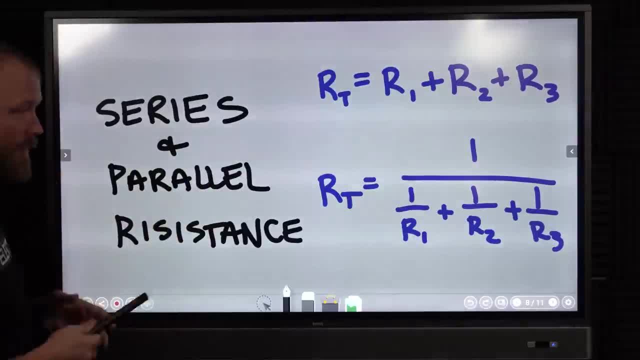 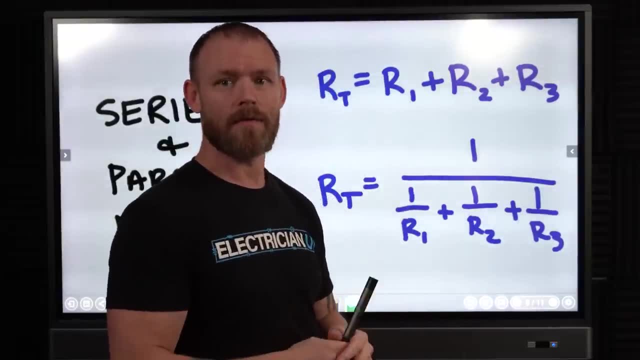 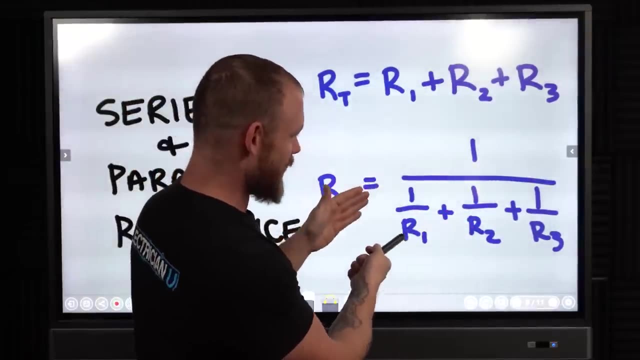 adding them all together. Where it gets kind of wonky is when we get to parallel resistance. Parallel resistance: you have to take the inverse of the sum of inverses. There's a different method: product over sum. We'll get to that here in the next slide. But it's a weird thing, right? So I just usually do like one divide. 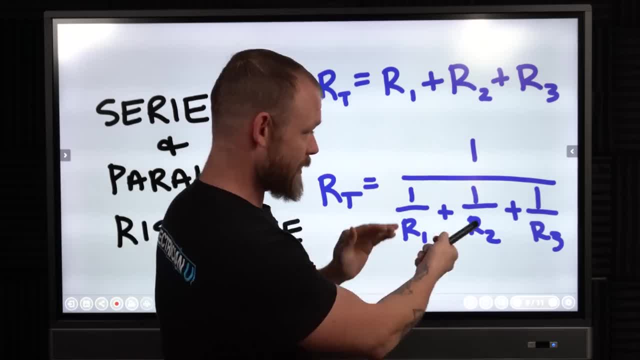 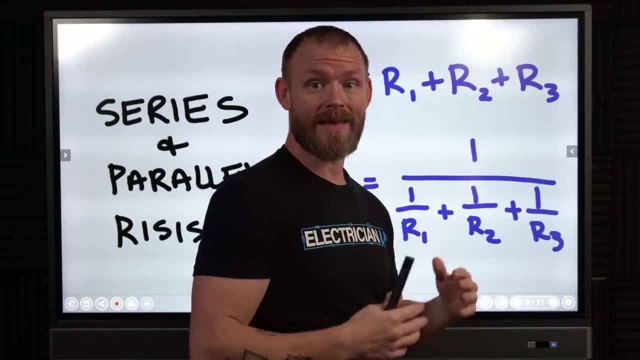 if it's a three ohm resistor or something I do- one divided by three plus one divided by two plus one, whatever, And you get that sum. and then you take one divided by whatever that sum is, and that's what you get. So you'll see the dramatic inverse effect on putting resistors. 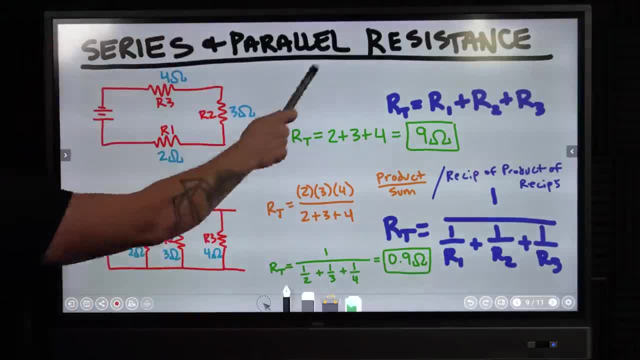 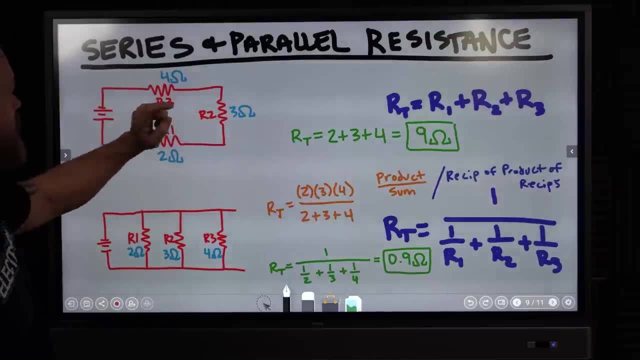 in a series circuit than you will in a parallel circuit. All right, So we're going to do series and parallel. So here we have a series circuit. We've got R1, R2, and R3.. There are three different resistors. R1 is two ohms, R2 is three ohms, R3 is four ohms. 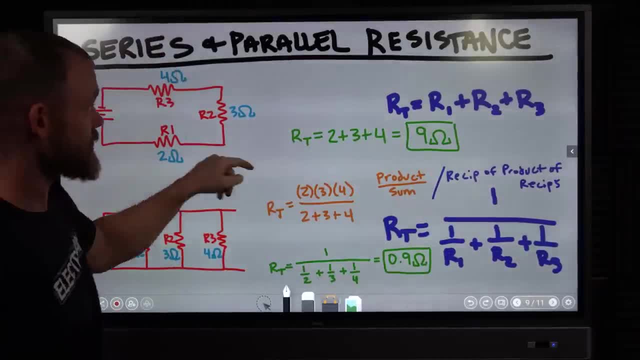 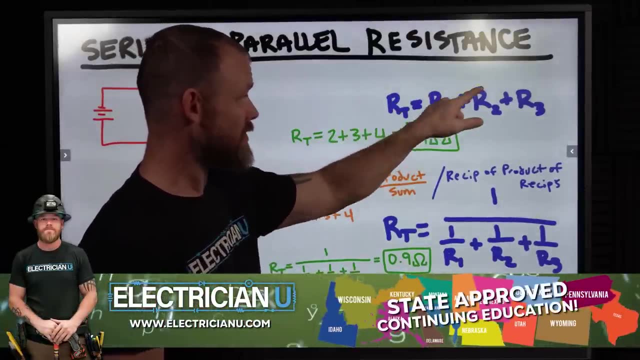 So we're doing series right, They're all in series. So we're going to do the sum of all resistances method. We're going to take the total resistance equals R1, R2, and R3 all added together. So we got two plus three plus four. two three, four, That's nine ohms of resistance. 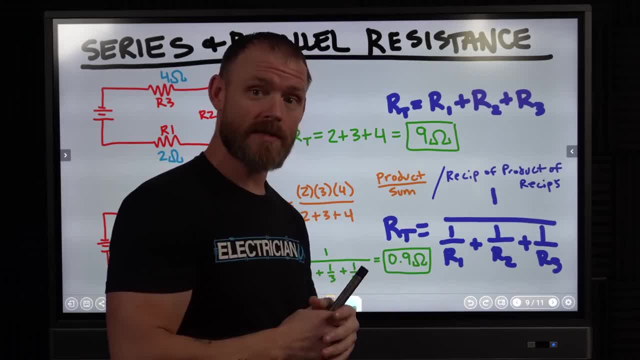 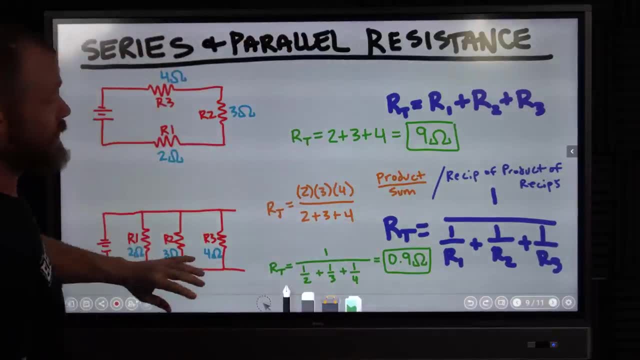 That's a lot of resistance because we have each one of them in series, So we're just adding more and more resistance to the circuit when we try to apply pressure or voltage. The next method is the reciprocal over the sum of reciprocals. So we were going to take 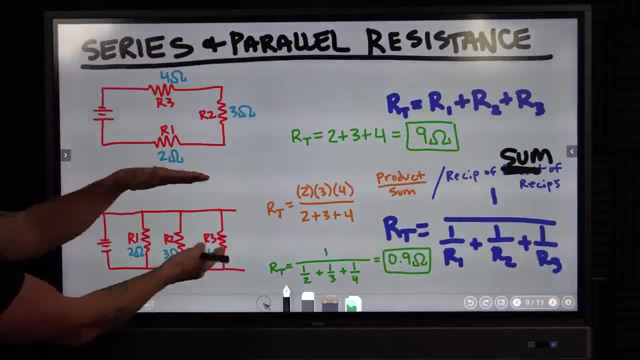 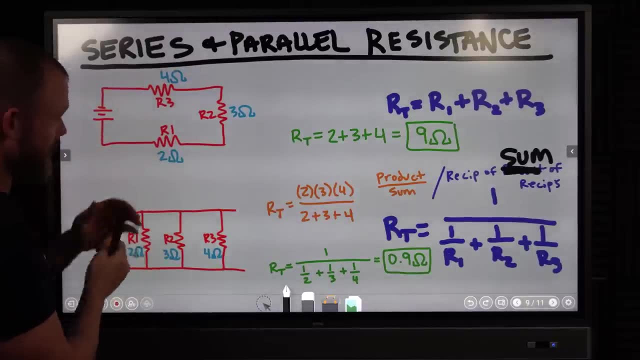 still R1,, R2, and R3, but in this circuit we're in parallel rather than in series. So we've got resistor one, two ohms still, three ohms still and four ohms still. We're just putting them in. 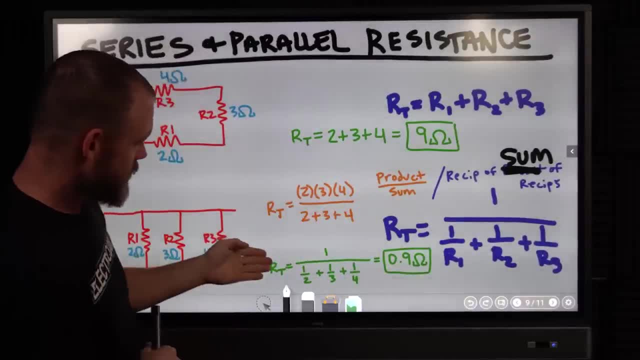 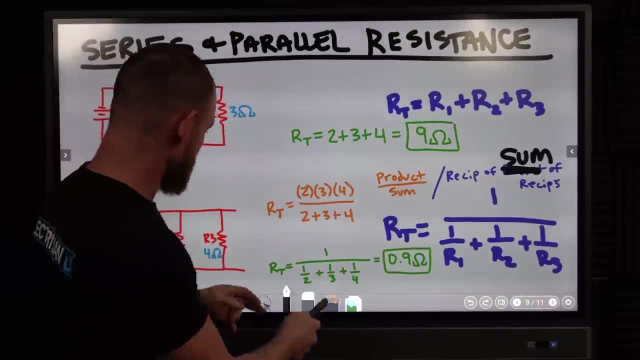 parallel in the circuit instead, And what we get is one over one-half ohms. Okay, Over one-half, right, Because the two plus one-third because of the three, plus one-fourth because of the four. We add all that up and then we take the reciprocal of it and it's 0.9 ohms. 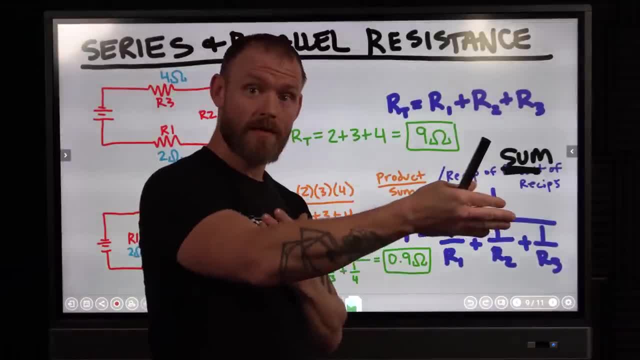 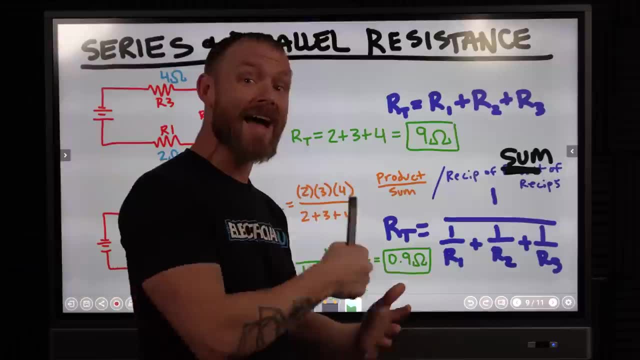 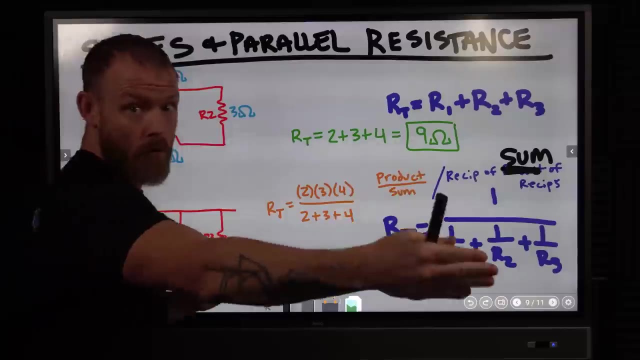 rather than nine ohms, So we actually get the inverse number. because it's going through. current is traveling through the circuit differently. It's not just one resistance being added to each. Current's going to go everywhere in this circuit, but there's nothing impeding it in a row in order. 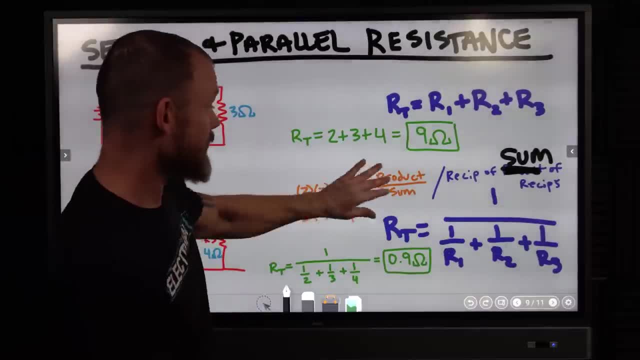 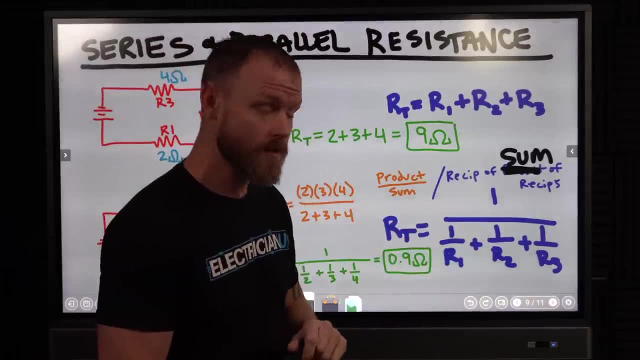 So you can sit and mess around with that and have fun if you want to. but I find an easier method of going about it is just to use the product over sum method. So you can do this craziness if you want to, but it's also possible to just do each one of the resistances times each other. 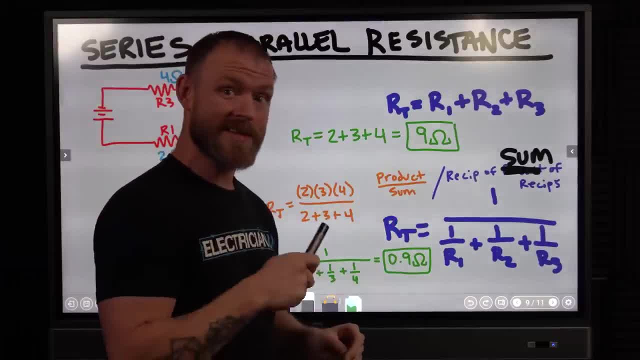 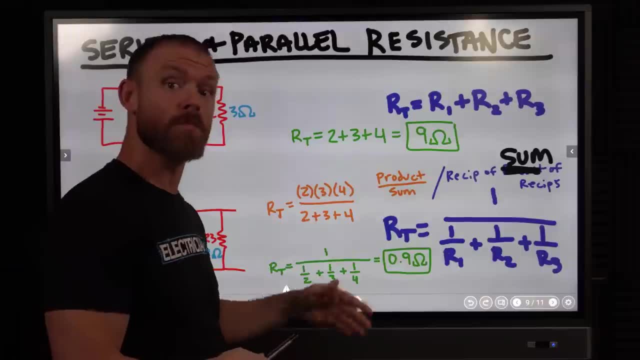 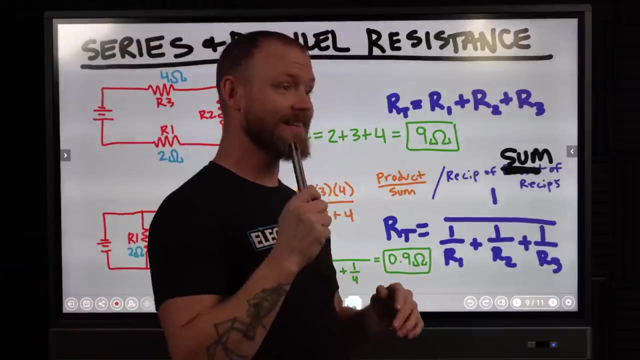 and then put over each one of the resistances added to each other. So the product two times three times four, the product over the sum to plus three plus four and you get the same exact number. So super helpful. You're going to run into lots of that once you start getting into taking. 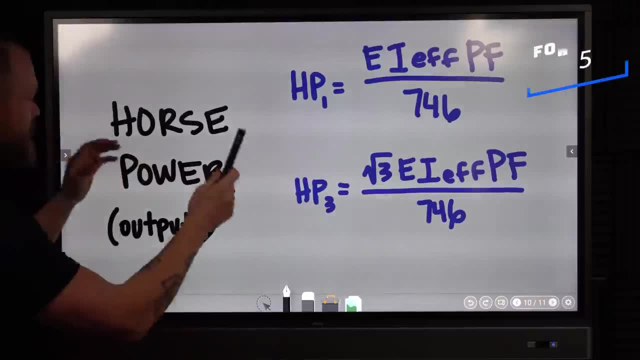 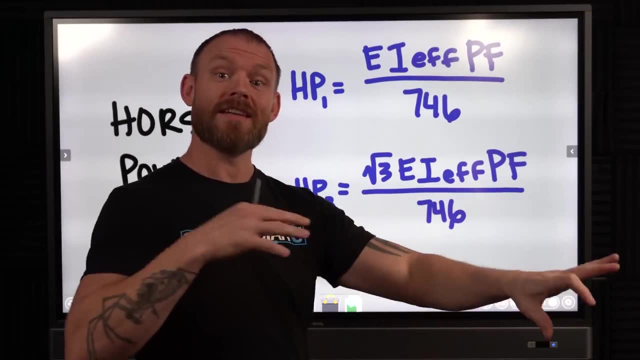 your electrical theory exams. So have fun. Last one we're going to talk about is horsepower, and we're specifically talking about the output of a motor. What is it going to put out, based off the conditions of the circuit and the conditions of the motor, not talking about just converting? 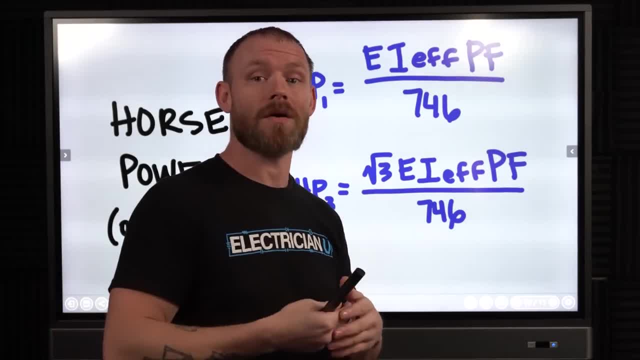 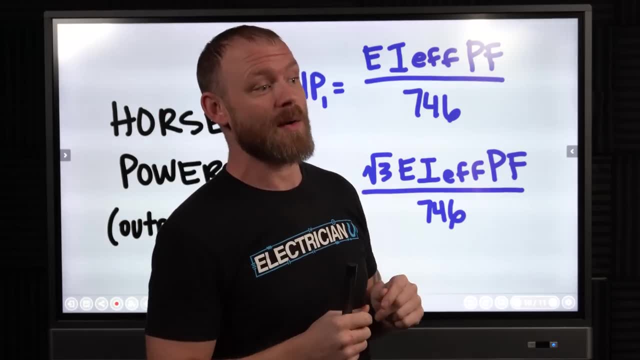 a watt to a horsepower, because one horsepower equals roughly 746 watts. That's another number. Just remember that. if you've ever tried to think of, like Hey, power motor, what does that produce? 746 watts roughly. But there's a lot more things to factor. 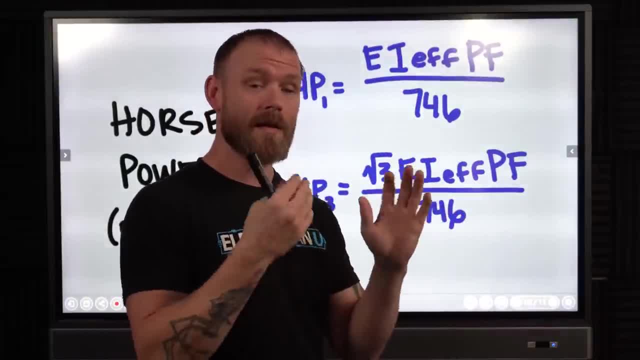 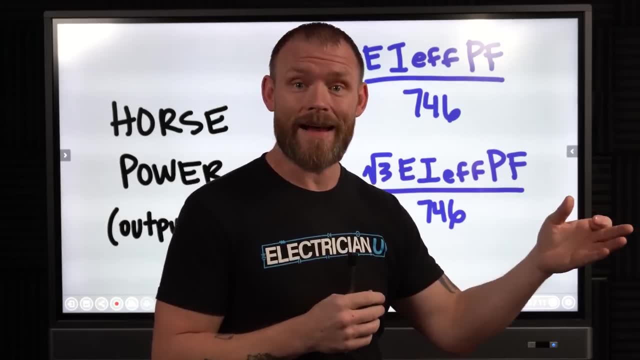 with a motor. Some motors are a lot more efficient than other motors. A lot of them have a rating on them and it'll say EFF and it'll give you efficiency of like 90% or 0.9.. So it's not 100%. 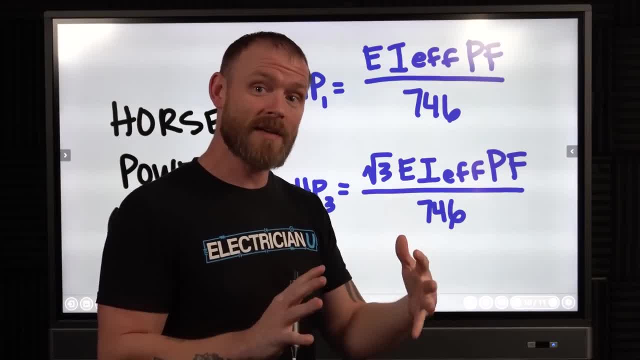 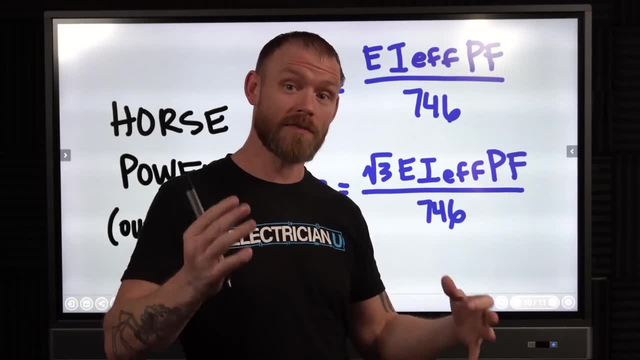 efficient? it's only 90% efficient, So that's going to change the dynamics of the output of that motor. Another thing is you could have a power factor problem. So you might be in a building that's got a lot of inductive loads, like maybe tons of motor loads. Well, the overall power factor 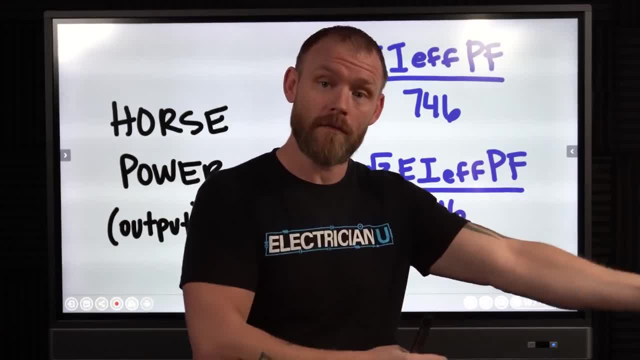 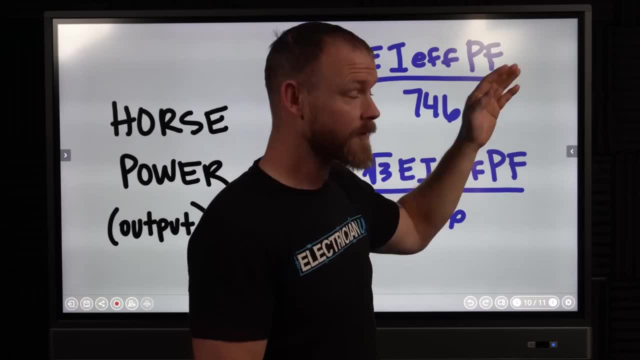 of that circuit is going to change the nature of the output of that motor. So we're going to be putting in voltage, amperage, the efficiency of the motor, the actual power factor for the circuit, and we're going to divide by 746, right, Because one horsepower equals 746 watts. So to figure out, 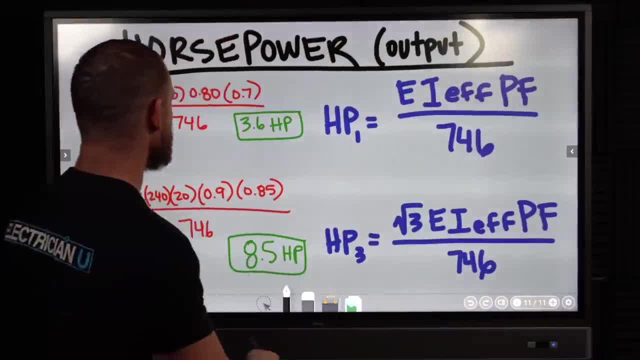 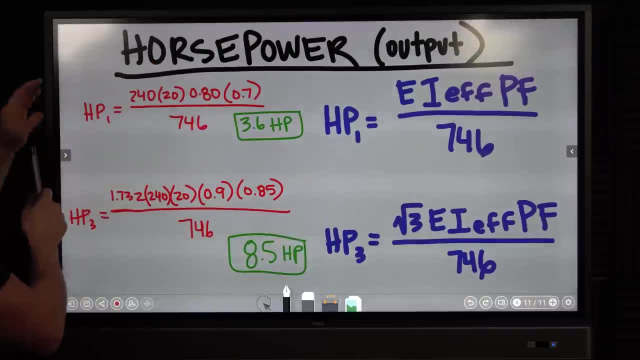 what the true horsepower of this motor is. let's look at an example. So we're going to be single phase, three phase. Again, we've got a motor that's got a lot of inductive loads, like maybe tons of the square root of three thing, right, Three phase. So let's look at a single horsepower motor. 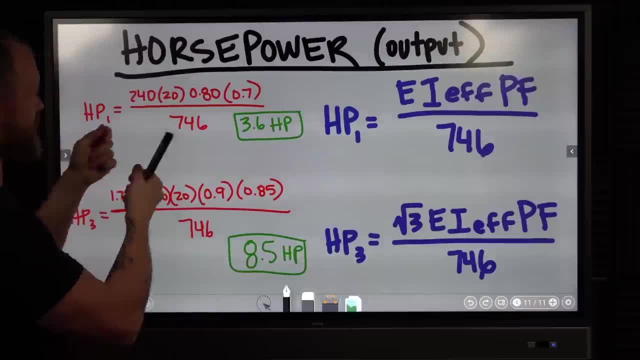 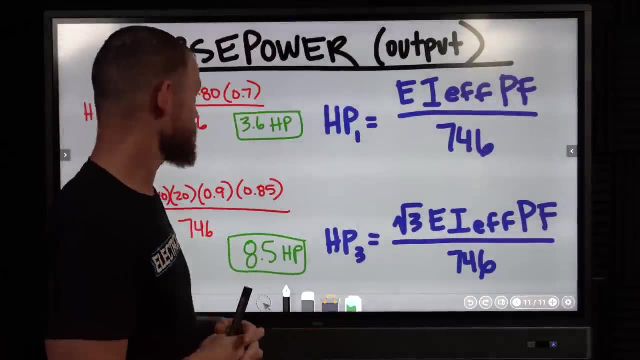 We're going to take the voltage times, say it's a 240 volt circuit, We've got a 20 amp motor. The efficiency on the motor actually says that it's only an 80% efficient motor. So not very great. And the power factor is kind of crazy at 0.7.. So unity power factor would be one If it's. 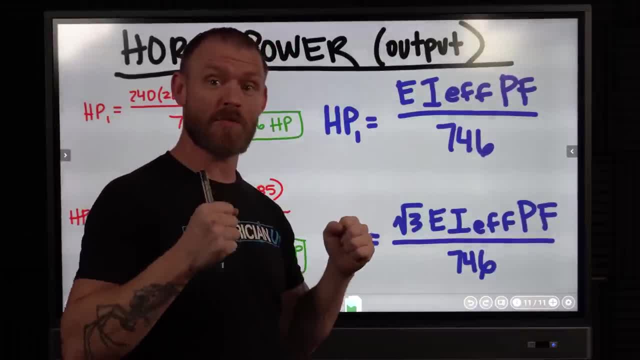 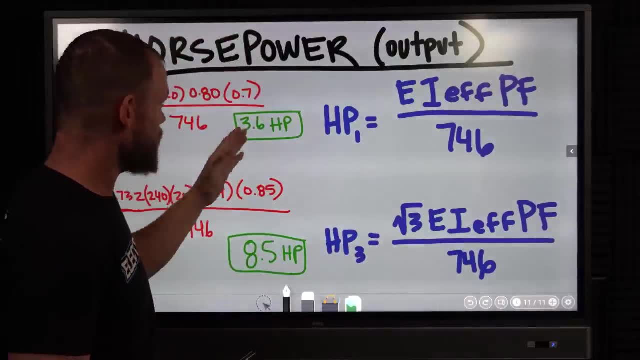 100% power factor. that means your voltage and your amperage. when you apply voltage, there's immediate amperage. There's no delay or lag reactance. that's happening, Then you're going to have one, but anything that's worse than that is going to be. 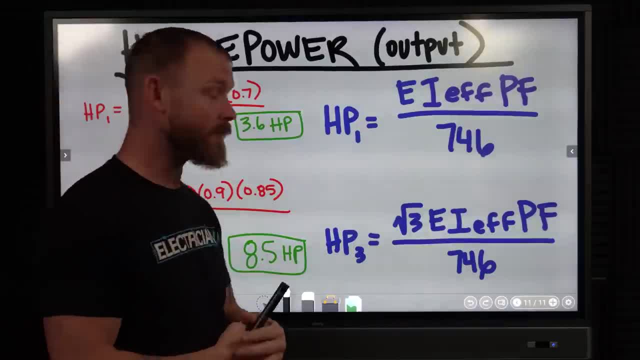 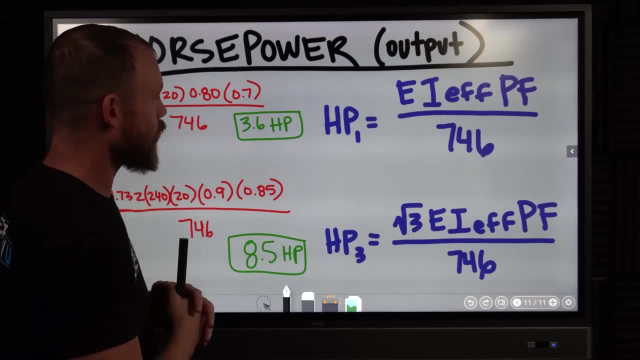 like below one. So 0.7 is a pretty terrible power factor. Then we're going to divide by 746.. So we do all the math- single phase horsepower- and we get 3.6 horsepower. Now that's not the actual. 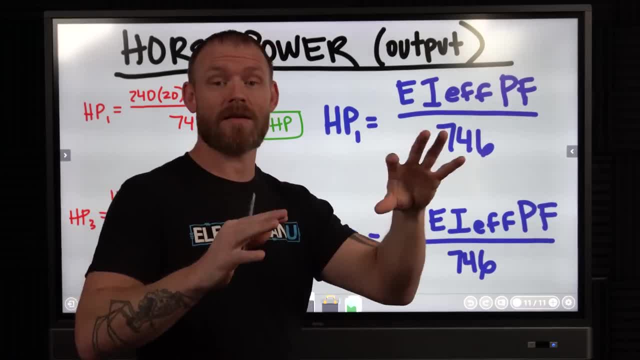 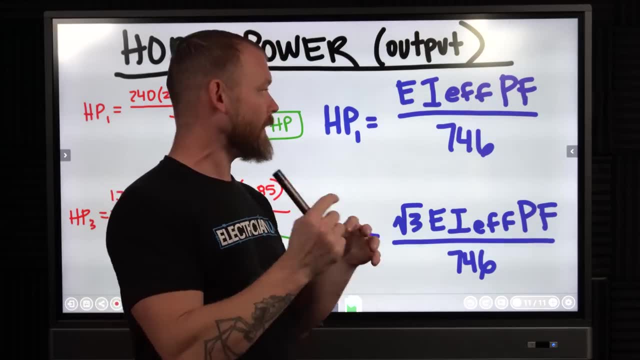 horsepower rating, sizing your conductors and doing amperage and all of that stuff. off of that You're going to use 430 in the national electrical code, 247,, 248,, 249, and 250.. And that's going to. 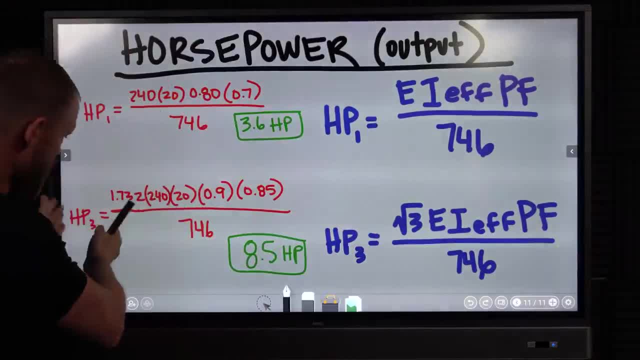